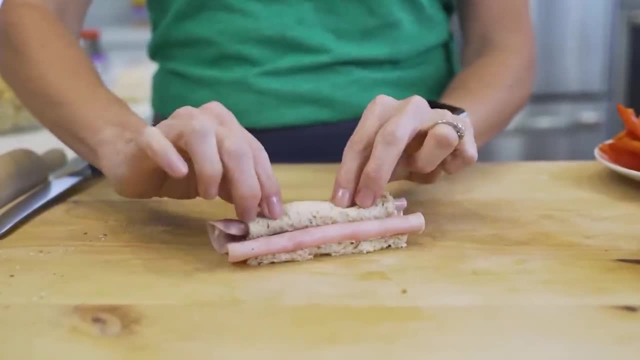 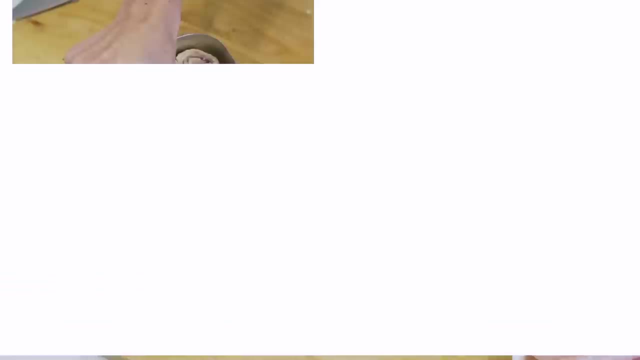 place your thin ham slices on top and then you roll it up like sushi. Once rolled up, you're going to slice it into small pieces and place it inside your bento box. Now all I have to do is fill the other bento compartments. 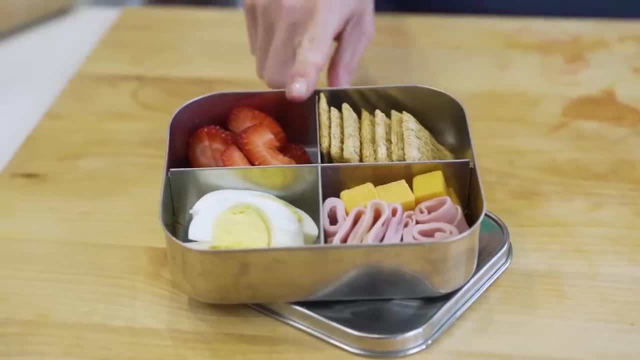 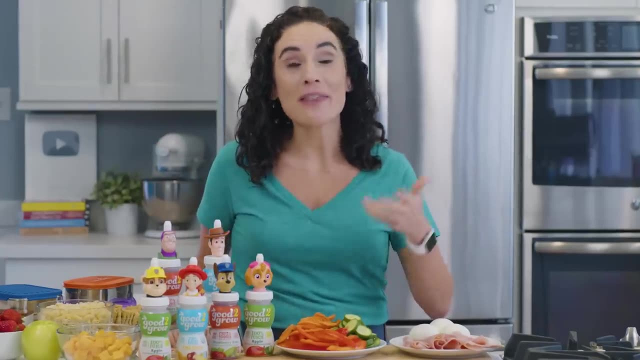 with fresh fruit and veggie. Now bento number two is for the kid that you're always thinking about how to get more protein into their healthy diet. The secret: Serve protein the way they enjoy eating in small pieces so they can munch on them. 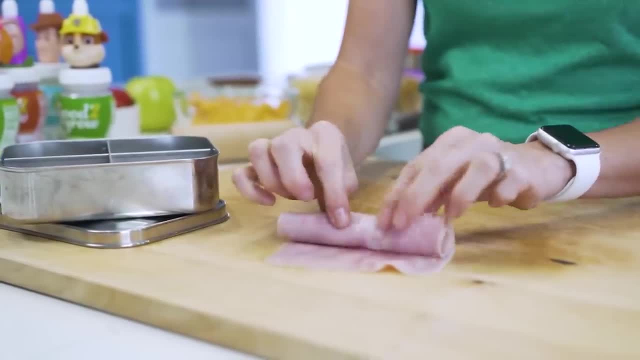 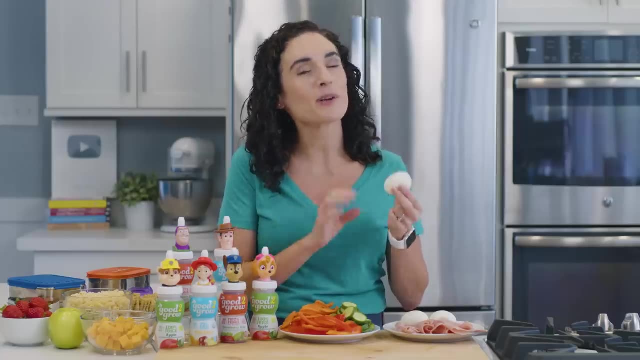 while they chat with their friends. I'm simply going to take some rolled up ham, slice it in small pieces, add some cheese cubes to the small compartment right here. I love hard-boiled eggs because they're perfectly portable and also more protein in the snack box. 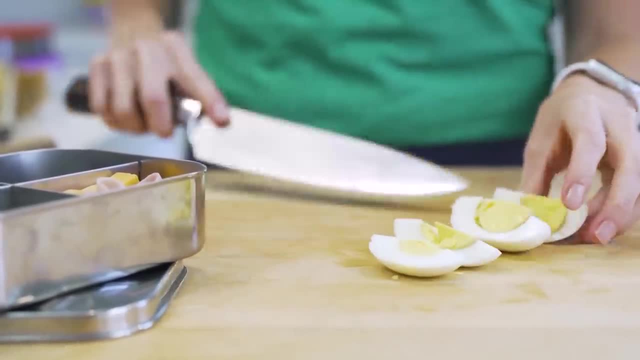 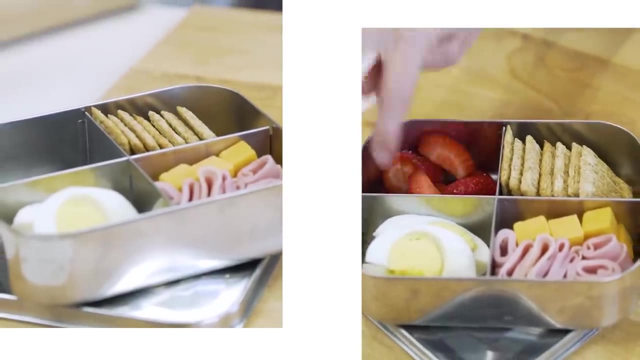 Of course you're going to precut it for your young kiddos by slicing it in half and then once again into smaller pieces. To this bento I'm going to add some diced strawberries and whole grain crackers. Now this next bento is for the grazing kid. 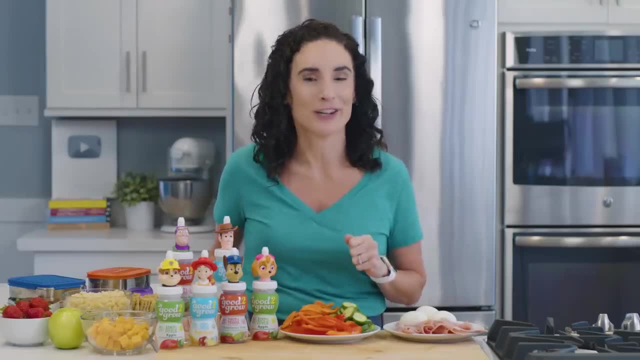 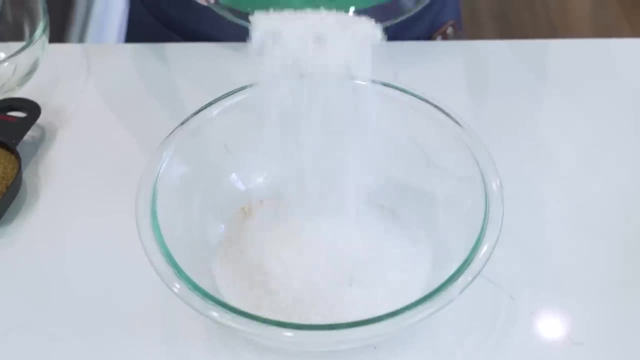 you know, the one that loves to snack and never quite sits down to finish a meal. I've got that one. For this one, I'm going to make some oatmeal bites by simply combining some oats, shredded coconut ground flax and a few mini chocolate chips into a bowl. 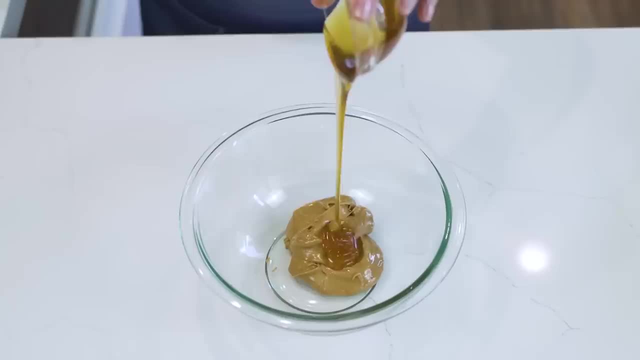 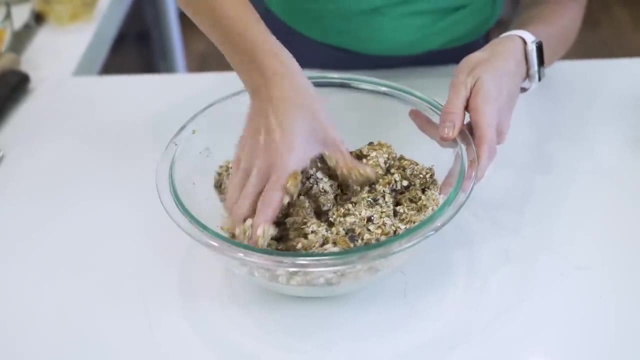 Now, in this separate bowl, I'm going to combine some nut-free butter with a little honey and add that to the dry mixture. With my hands, I'm simply going to form small, bite-sized balls. The great thing about these is that they can be stored in the fridge for up to a week. 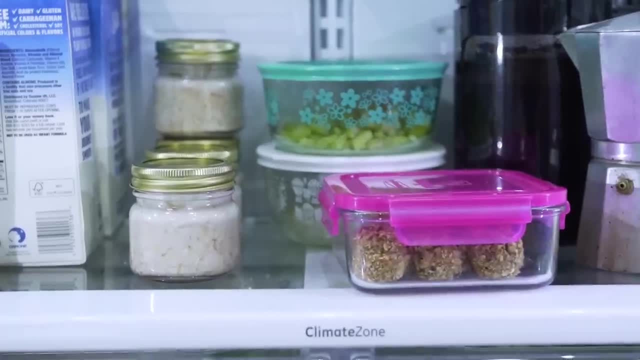 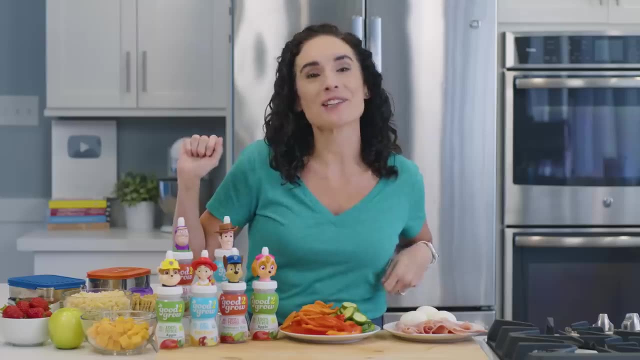 and, being that they are nut-free, they are safe to send to school. Place a few inside the bento along with sliced hard-boiled egg, sliced apples and some veggies. This next bento idea will encourage you to use up leftovers and turn them into another meal. 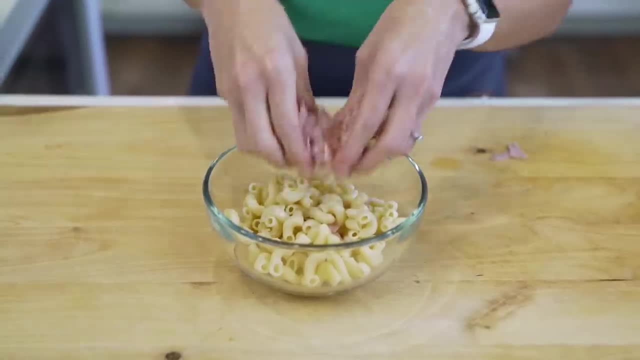 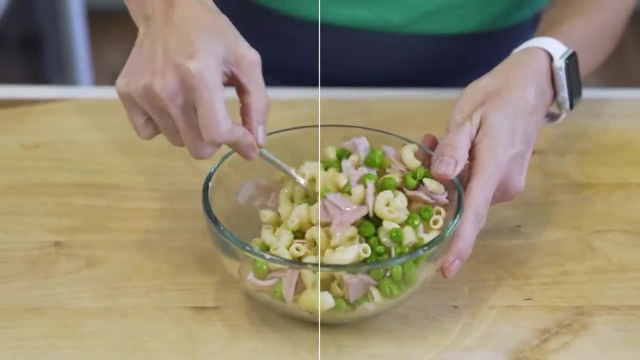 like this elbow macaroni leftover from dinner that I'm going to combine with some diced ham, some frozen peas and a little olive oil in a bowl. It's super easy and fast. Along with the pasta salad, I'm going to send some diced strawberries.